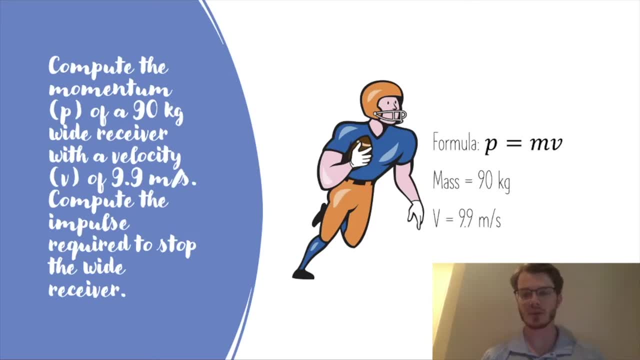 mass is 90 kilograms and our velocity is 9.9 meters per second. When we add this into our equation, we're going to get our momentum to be 891 kilograms per meters per second. So for our impulse we are actually going to have the same impulse as our momentum. 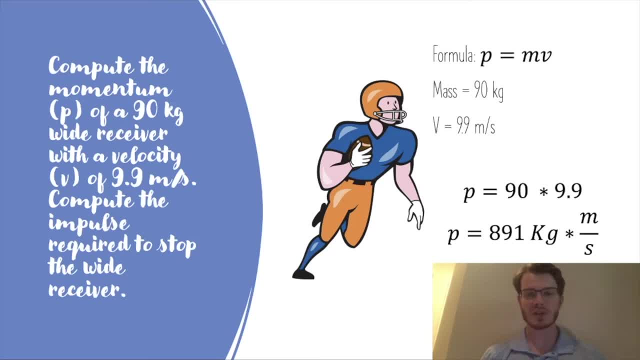 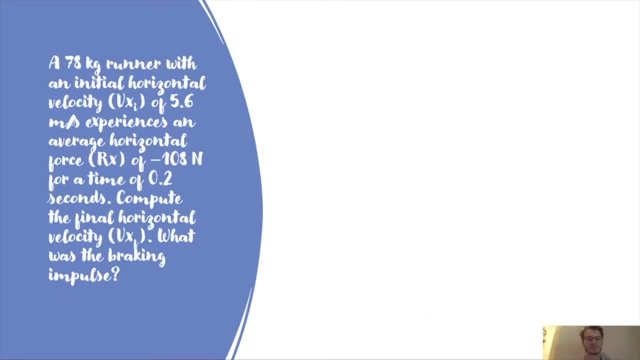 because we are wanting to stop the wide receiver. So in our laws of motion we have to have that same force to have an object come to rest. So our impulse is actually going to be 891 newtons per second. For our next question, we have a 78 kilogram runner. 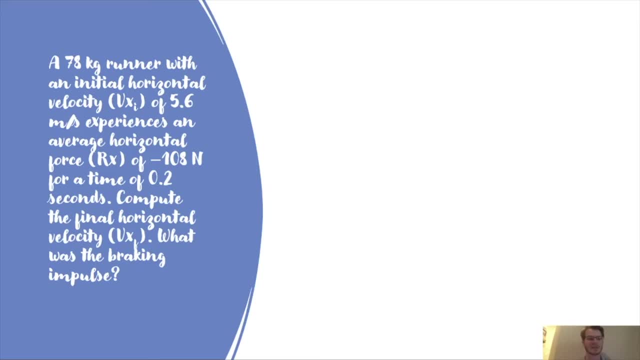 with an initial horizontal velocity of 5.6 meters per second, He experiences an average horizontal force Rx of a negative 108 newtons for a time of 0.2 seconds. Compute the final horizontal velocity and what was the breaking impulse. 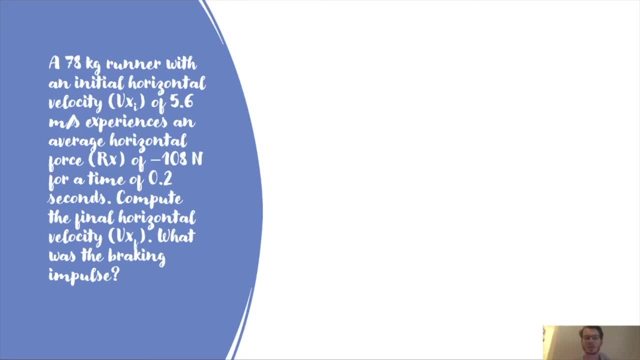 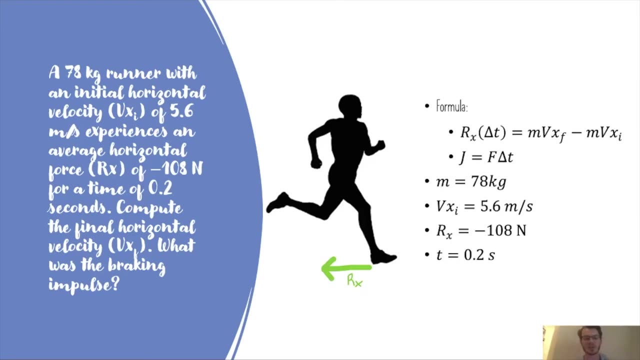 As always, we are going to draw out our picture, write out our formulas and write out our knowns. Here you can see in my picture I have the horizontal reactionary force pointed to the left, as it is a negative number of 108 newtons. 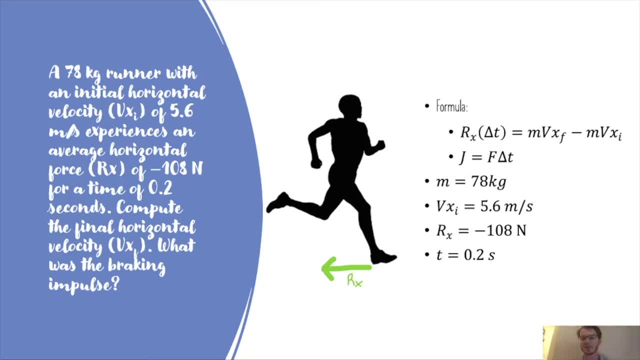 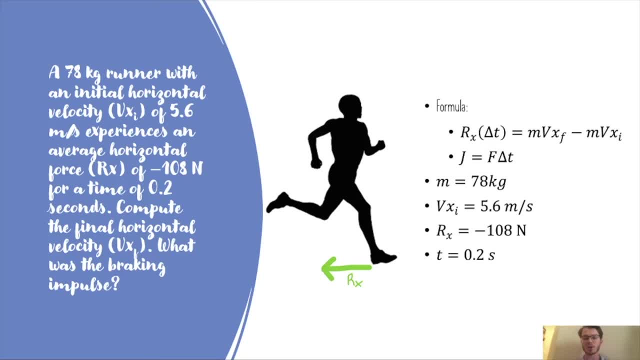 And our horizontal reactionary force of negative 108 newtons for a time of 0.2 seconds. We can then manipulate our formula to solve for our final velocity and then add in our knowns to where we get negative 108 times 0.2.